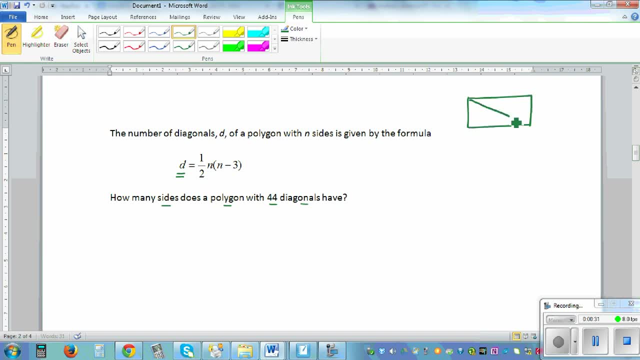 this is a rectangle, it has four sides and it has got two rectangles, two diagonals. So in this case you've got, let's say, n is four, diagonal is two, two diagonals, and so on, If you have a say, pentagon. 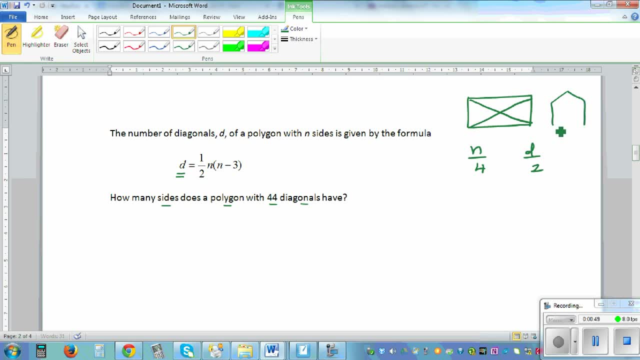 say, a pentagon would look like this. It's not exactly a pentagon, it's not regular pentagon. So you've got one, two, three, four, five diagonals. So if you've got in the pentagon, you've got five sides and you've got five. 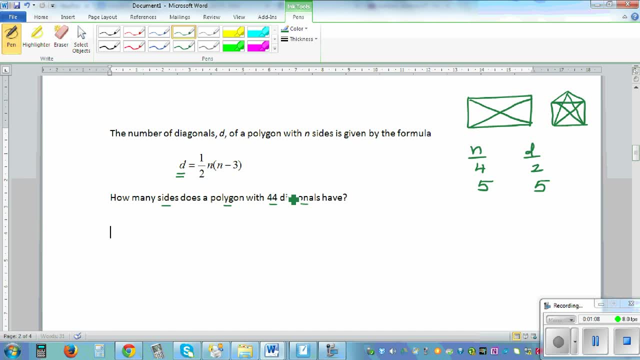 diagonals. So the question is, if D is 44, how many sides does this have? So let's put D as 44.. So if you put, 44 is equal to half times half, n times n minus three. So I want to get rid of this half. so 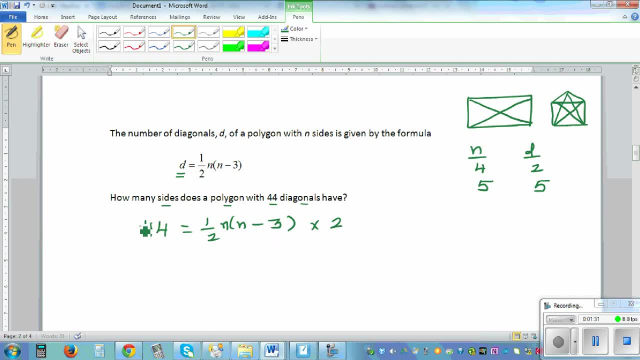 I'm going to multiply by two to this side, So I also multiply two to this side, So this two and this two gets cancelled. So this is: 88 is equal to n times n minus three. Okay, so this is expanding this out. You can say: 88 is equal to n squared minus three, n Now taking away 88 from this side. 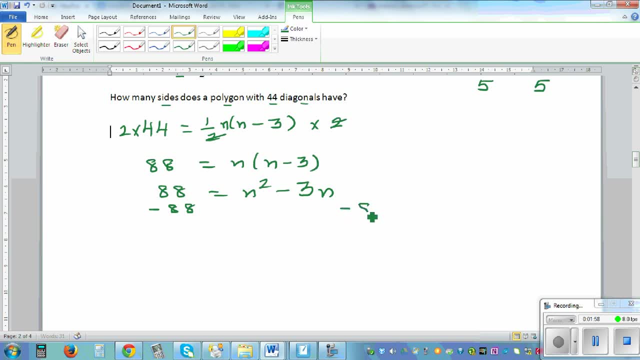 if you take away 88 from this side, you can take away 88 from this side. So this becomes a quadratic equation. So you can say: zero is equal to n squared minus 3n minus 88.. So let me write this in a general quadratic form. So this is n? squared. 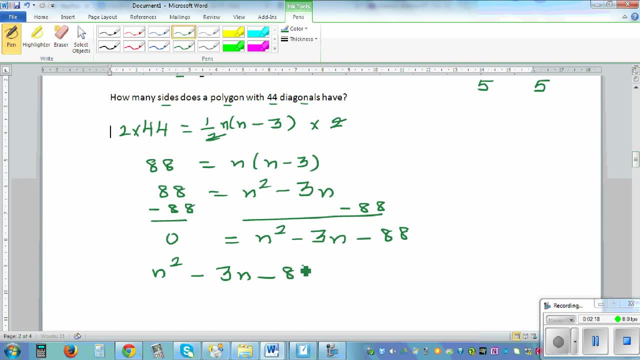 minus 3n minus 88 is equal to zero. So now let's put them in two brackets. So this is well, you have to, as you go, n squared to start with n and n. The two factors of 88, which gives you minus 3, is minus 11 plus 8.. 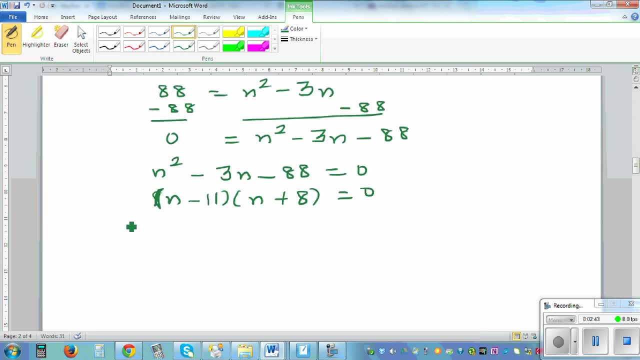 Okay. so here we can say: if you set each of them equal to zero, I can say n minus 11 is equal to 0, or n plus 8 is equal to 0. So you can say n is equal to 11 or n is equal to negative 8..